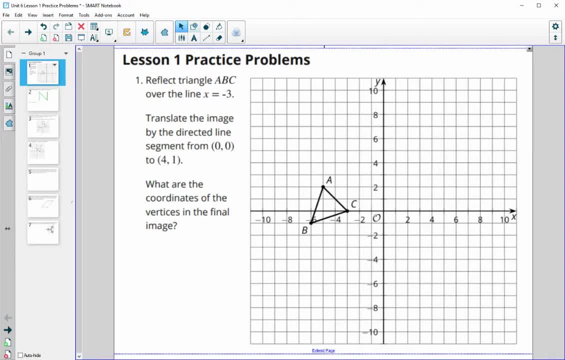 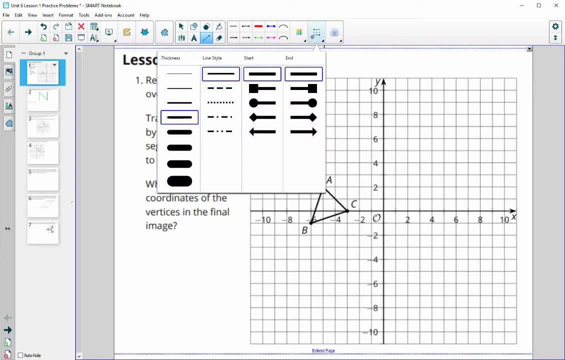 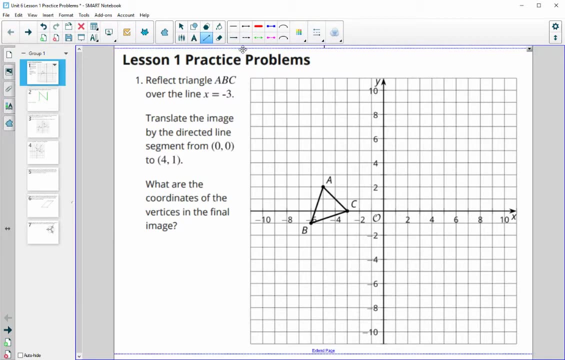 Let's take a look at the practice problems for lesson one in unit six. So this one asks us to reflect triangle ABC over the line x equals negative three. So let me get that line on here first. All right, so we'll put the line x equals negative three on here, And then we 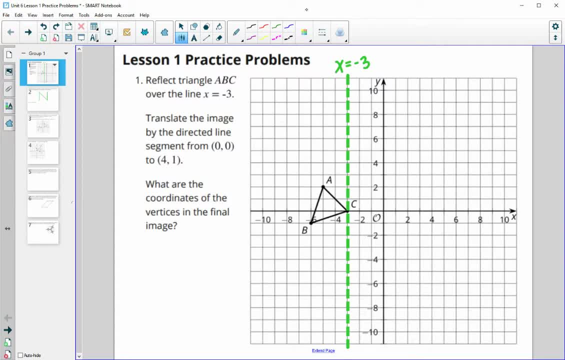 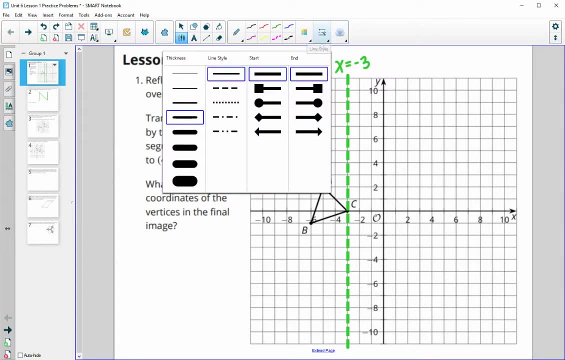 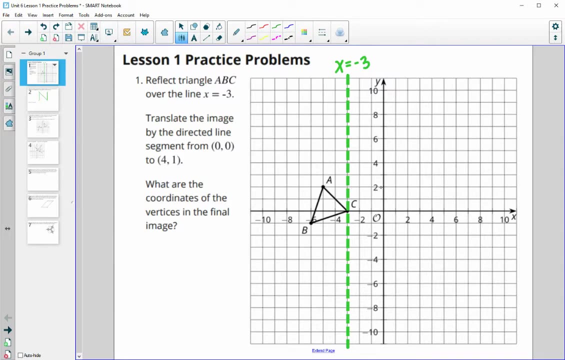 are going to reflect this triangle over that line. So that means that all of the points are going to reflect to an equal distance to the other side. So we'll count how far a is away from the line. So it's two points away from the line to the left. So we'll go two points to the right. 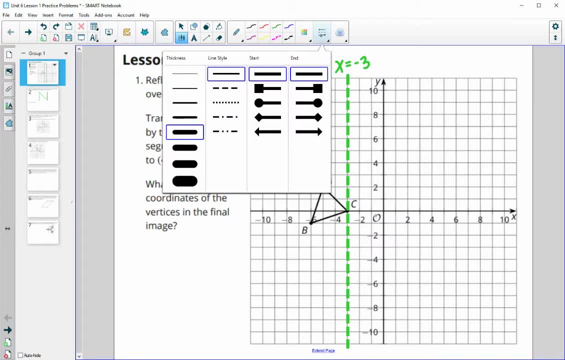 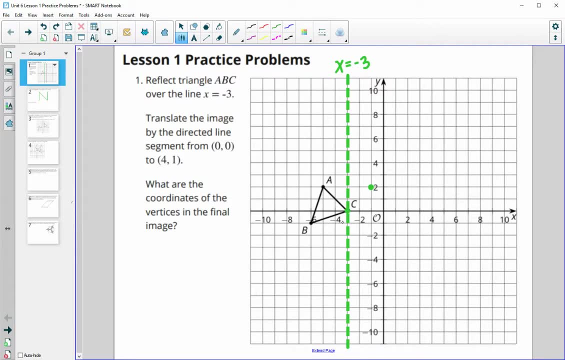 Whoops. So we'll go: two points to the right of the line, So one, two to the line, So one, two off the line. C is on the line, So it will stay. B is one, two, three to the right. 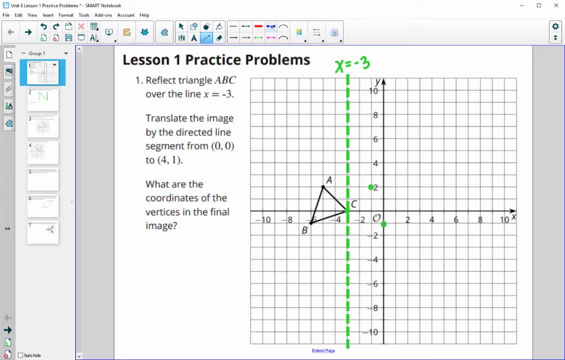 So we will go one, two, three to the left And then so I'll just connect those. So here's our second line, Here's our second part of the. here's our image with the reflection. So that was this first part, And now we will go ahead and translate the image by the directed line segment from: 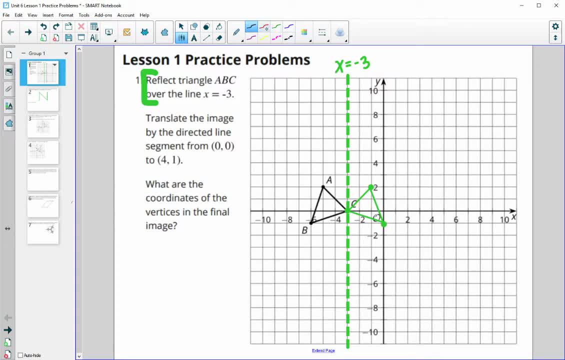 zero. zero to one, four. So you can look at remembering that the x movement, okay, is to the right or to the left, So that's zero to four, So that's going to be four to the right, And then the y movement is going to be up or down, So this is one up, So we're. 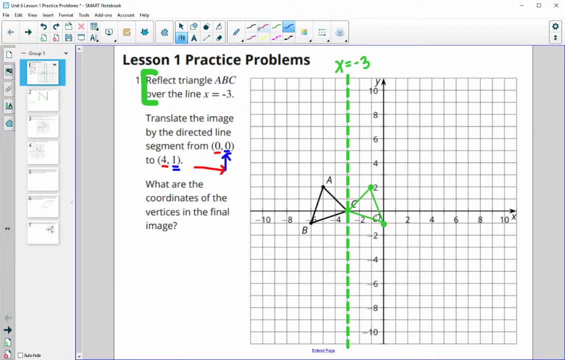 going to go four to the right and one up. with this You can also- if that's hard to figure out from the points- you can also draw the segment. So if you want to draw the segment on zero, zero to four, one, and then you can count the horizontal and the vertical movement. 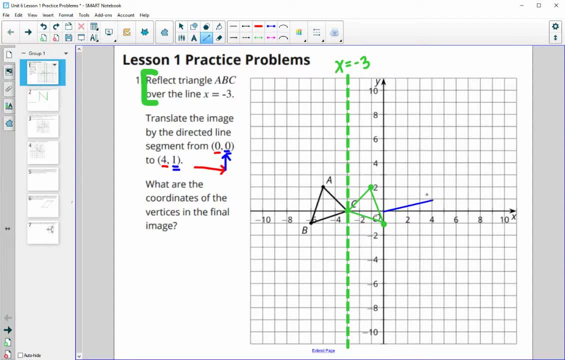 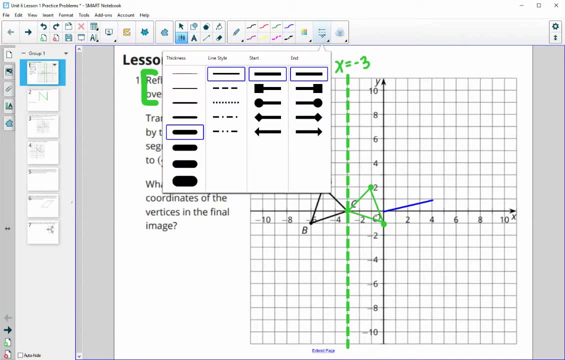 that way, So you can see that that's four. So we're going to go four to the right and one up, And then you're just going to move that from each of your points. So we'll go from a prime or from this new a, so one, two. 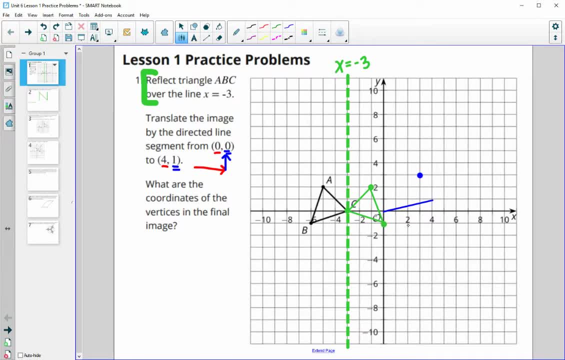 three, four up one, one, two, three, four up one, one, two, three, four up one. And then we can connect that. And then it wants to know these new points, the ordered pairs of these. So this is our. 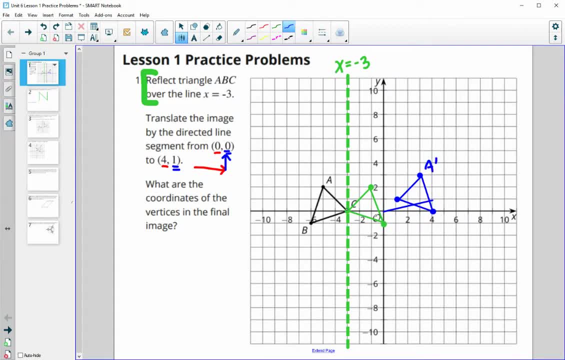 new a, so this is a prime. This one was C prime, So B flipped to here, So this one was B prime, So a prime is the. is the ordered pair: one, two, three. one, two, three, so three, three. 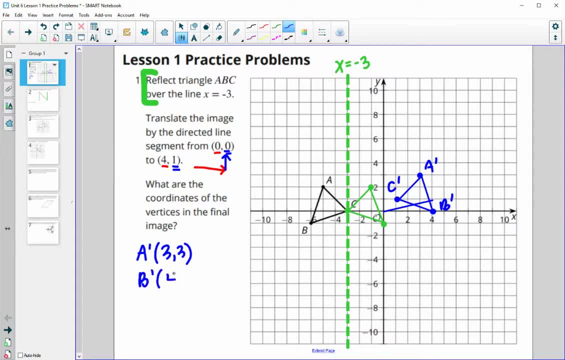 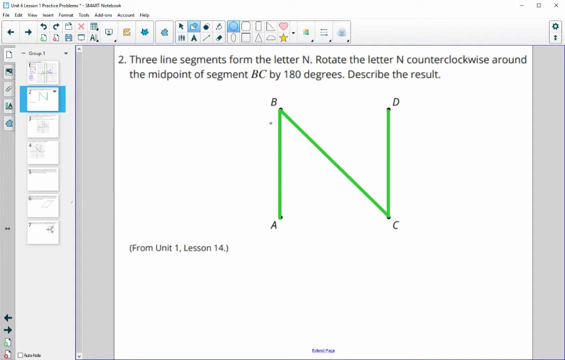 B prime. B prime is at four zero And C prime is at one one. Okay, number two gives us three line segments that create the letter N. and then we want to rotate this N counter clockwise- Okay, so to the left or backwards. okay, this way. 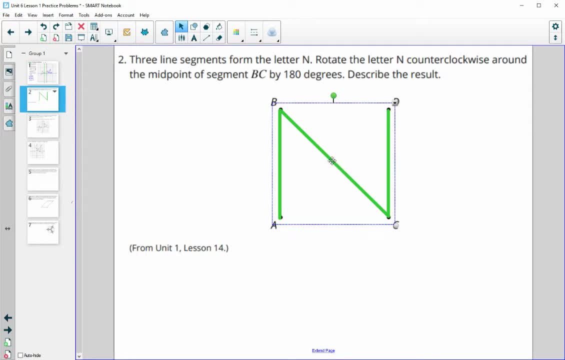 Around the midpoint, middle of this segment. so this point will stay the same and then everything will rotate around it by a hundred and eighty degrees and then describe the result. so we're gonna rotate this counterclockwise, so this is 90 degrees and then this is 180 degrees, so that it just landed on itself would be the 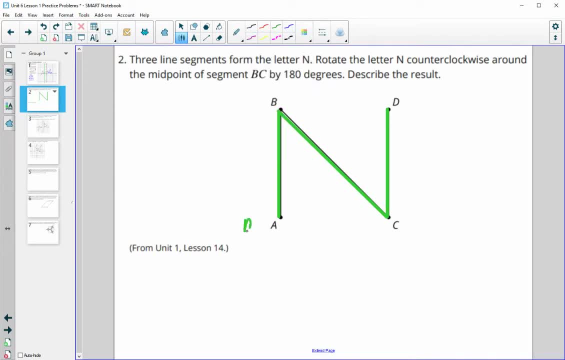 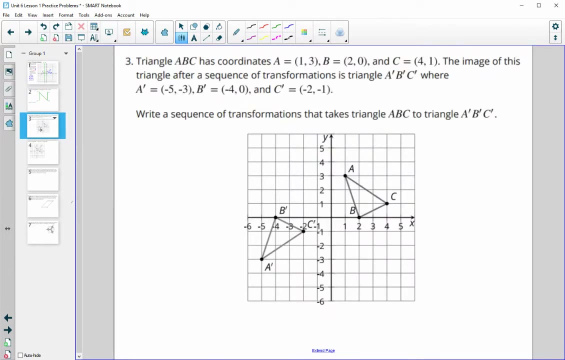 result there. so D landed over here. so D prime is on a, C prime landed on B, a prime landed on D and B prime landed on C, so it just rotated on itself, all right, um, this one has two triangles that are plotted for you, so ABC at these points. 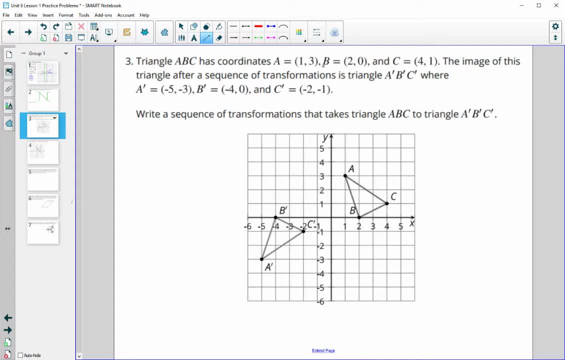 and a prime, B prime, C, prime at these points, and it wants us to give a sequence of transformation so you could have multiple different sequences of transformations here. there's not just one correct answer. so let me draw this on and then, instead of doing the letters, I'm just gonna change the colors of these. 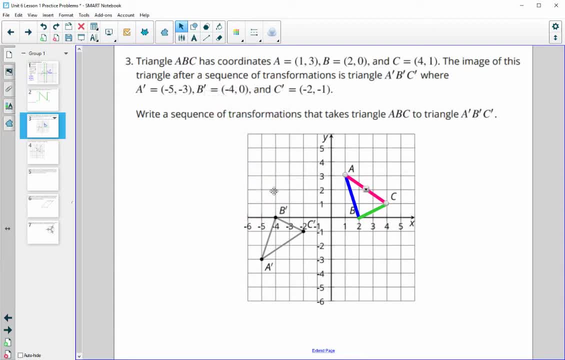 and so that we can see where they move to. so then let me put this one so a C I had as pink, so let me do that BC green and then AB blue, so that as we move this around we can kind of see if it's what's gonna land on its side. 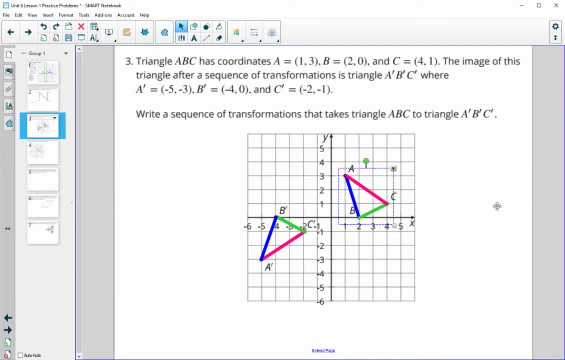 All right. So one thing you can do is one option would be to move B to B prime. So that would be a translation. So let me write this out as we do it. So translate ABC, So translate triangle, ABC along. And now this one: we just moved to the left, So we went 1,, 2,, 3,, 4,, 5,, 6 units to the left. 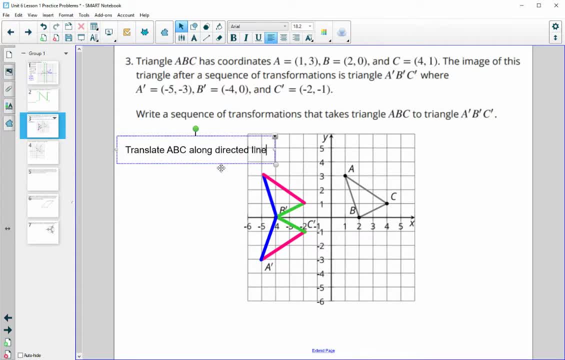 So translate ABC along directed line, segment 0, 0 to negative 6.. So we move it just 6 units to the left. Okay, so that got B on to B prime, So then we could rotate. So now we want to get this one of these: either the blue segments on top of each other or these green ones. 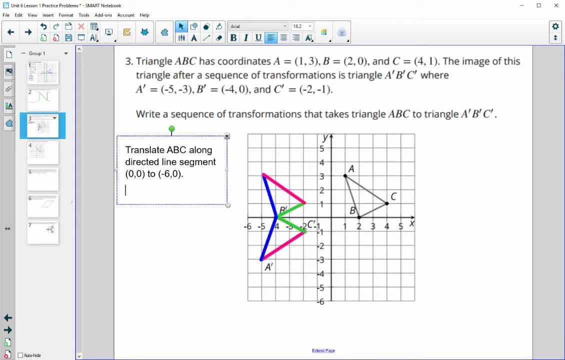 So I'm going to rotate the green, So this is point C. So then rotate ABC around Point B, So B is the center of rotation, or B prime, So around point B, prime, clockwise. So let's do then rotate triangle ABC clockwise around point B until C, this point until C coincides with C prime or lands on top of C prime. 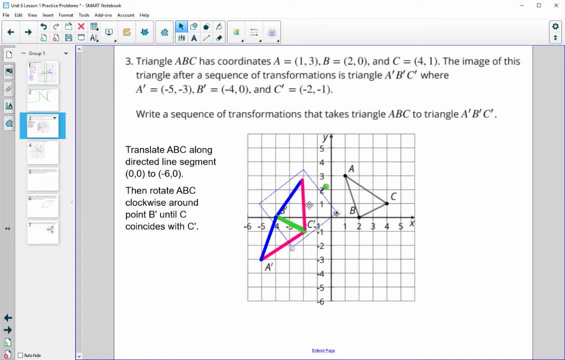 So we're just going to rotate and B will stay in place. So we'd be rotating around B until C lands on C prime. Then our final thing would be to reflect- Okay, then reflect ABC over line segment B prime, C prime. 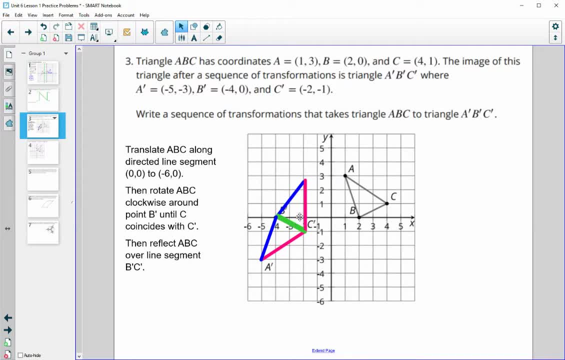 So that would get you there. That would just flip that over. Okay, that would be one that would get you there. Multiple others, So we can see If we have some others that we could do. So we know that we needed to do some type of reflection. 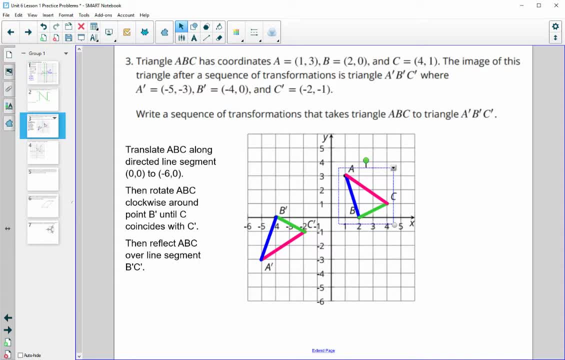 So maybe let's try reflecting first. So I'm going to just reflect this left and right, Okay, so I'm just going to reflect it and maybe I'll just reflect it over the Y axis. Okay, so, reflecting it over the Y axis. 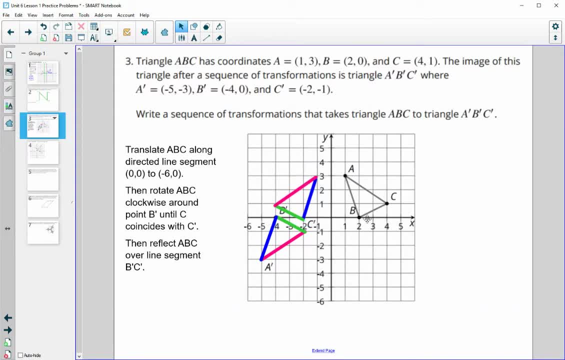 So this point A moved over one. B was two away, So B prime is going to be two away. C was four away, So C prime is going to be four away. And then we could look at translating, So just trying some different things here. 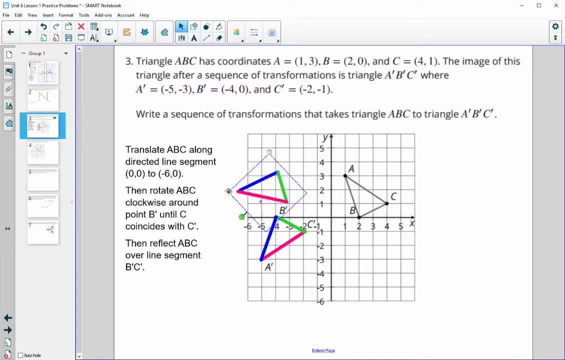 So could translate there And then again do a rotation around. Okay, so it could do something like that. So some type of, like I said, reflection. So I reflected over the Y axis, then translated to get the points together, then rotated. 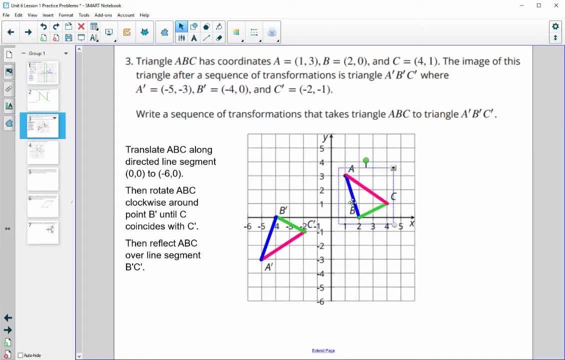 Okay, let's see if there's what else we could think about doing Could reflect over the X axis. So maybe we could reflect it over the X axis. So if we did that, point B would stay the same. So reflect over the X axis. 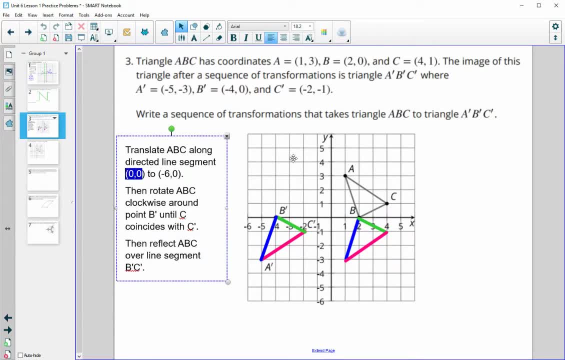 So let me, Let me write this one out, because this one's going to be just a couple of moves here. So reflect, oops. reflect A, B, C over the X axis. Then we can translate, because now we see it's like right, in order. 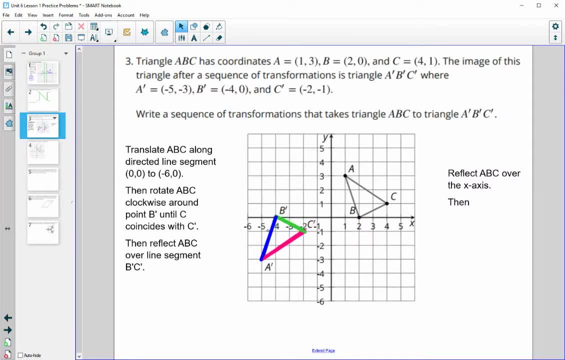 So now we could translate it six units to the left and it would land right on top of that. Okay, so then Translate triangle A, B, C by directed line segment: negative six, zero, or sorry, zero, zero to negative six zero. 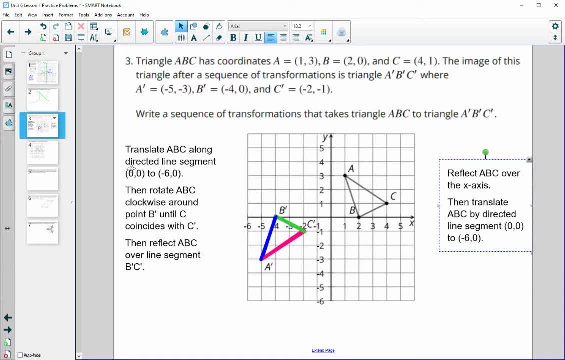 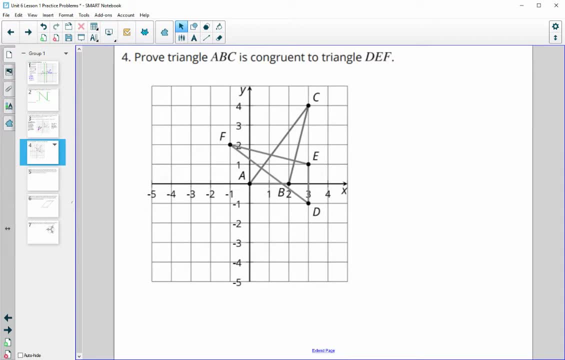 So there's a few options Again. I'm sure there's multiple more that would work as well. That's just a couple. All right, Prove that these two triangles are congruent to each. So this is going to be using side side, side side angle side or angle side angle. 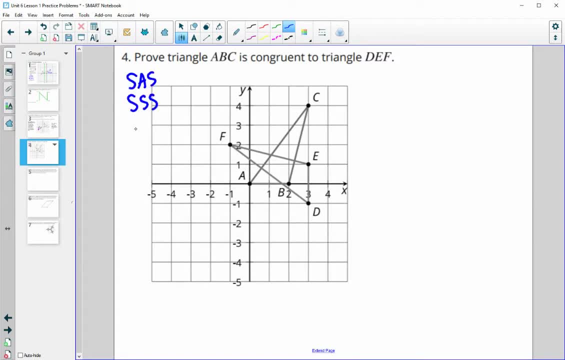 So those are the ways that we proved triangles were congruent, So it's likely that this one's probably going to be the easiest when you don't have a right angle, So you don't have a horizontal and a vertical line that you can see and you're on a grid. 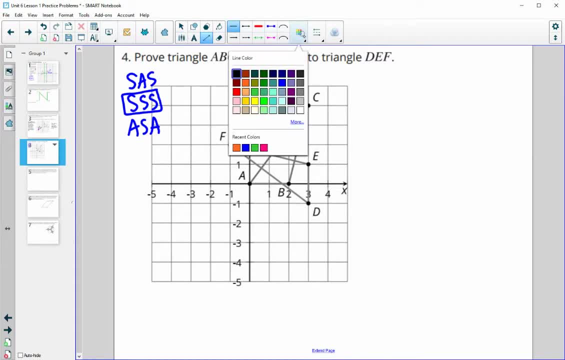 So we'll go ahead and prove that these different segments are congruent to each other. So let me highlight some here. So AC, So I'm going to find the length of AC and I'm going to do Pythagorean theorem, So I'm going to draw a right triangle off to the side there and then prove how long AC is. 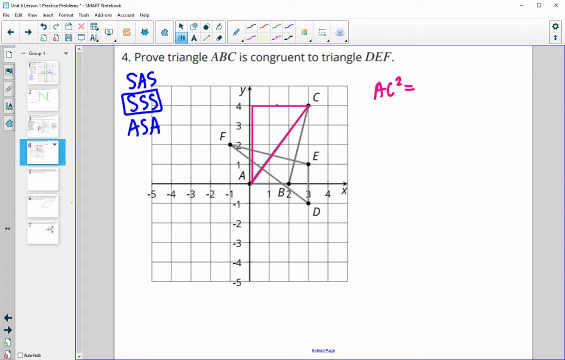 So AC is the hypotenuse, So AC squared equals. and then count this as three, And then count this one as four Equals, three squared Plus four squared. So AC squared is equal to nine plus 16.. Which is 25.. 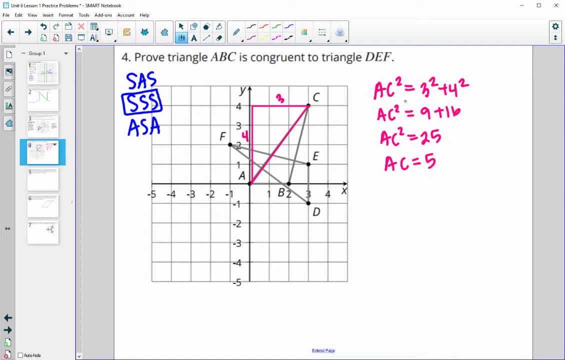 And then square root, that So we get AC is five. So then I'm going to get rid of these triangles off to the side as I prove different side lengths so that it doesn't get too messy, And then now do this next one. 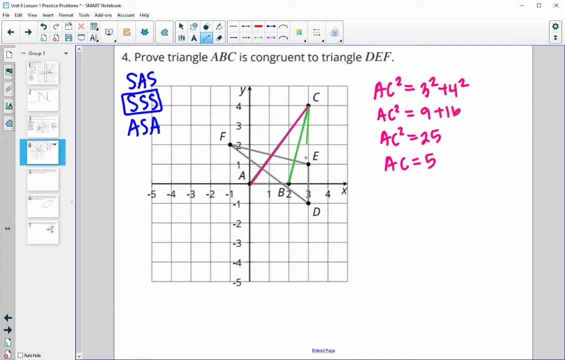 So this one Here, So side BC, So the triangle that would go along with this one, or the right triangle that would make that the hypotenuse would be here. So we've got BC Squared equals and the legs here are one. 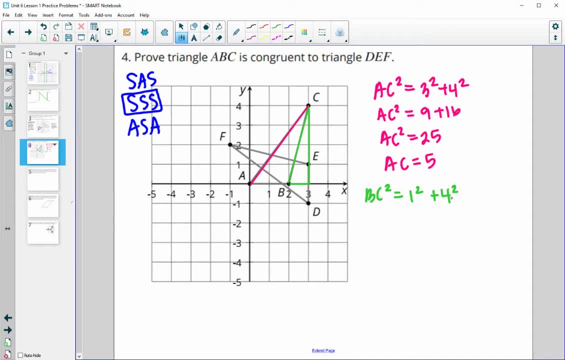 And one, two, three, four, So one squared plus four squared. So BC squared is equal to one plus 16. Which is 17. So BC is going to be equal to the square root of 17.. So again, I'll get rid of this. 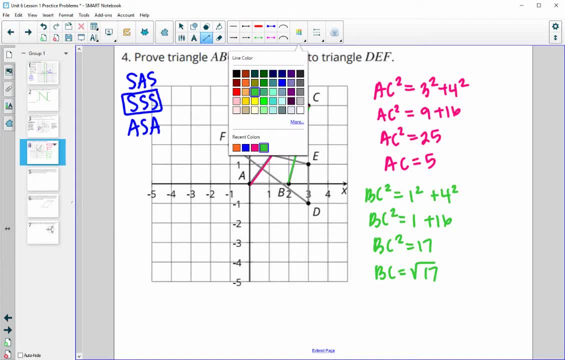 And then AB. here we can just count Since it's horizontal, So this one will be able to just count. So AB is equal to two. So there's the lengths that we have. So then we need to go and look at that for the other. 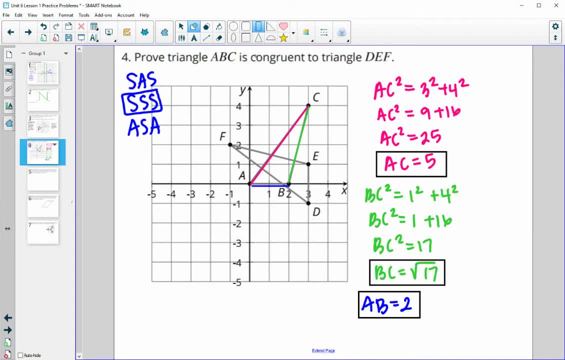 The lengths in the other triangle. So we'll go ahead and look at the one that would be like this pink one. So here- And if I do that and I draw this right triangle on, that would have that as the hypotenuse- We can see that we again have legs of three and four. 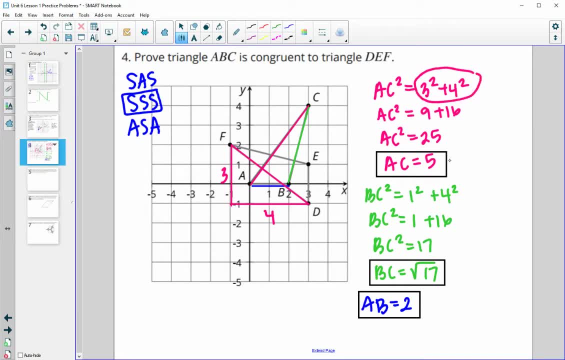 So it's going to be these exact same numbers, So FD is also Going to equal five. And then when we go ahead and look at FE, So here's FE. The triangle that would go with FE would be one And four for the legs. 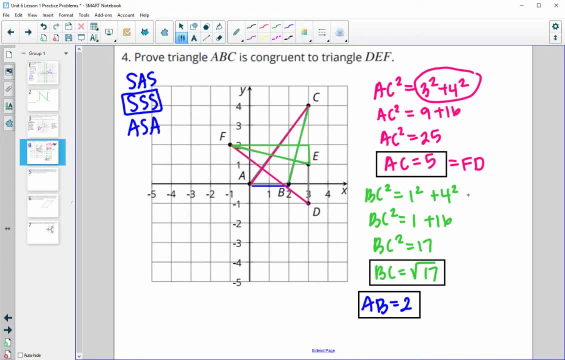 So again, that one's going to be equal to this one, It has one and four as the legs again. So we're going to go ahead and look at that. And then, when we go ahead and look at So, when we do the Pythagorean theorem, we're going to get square root 17 again. 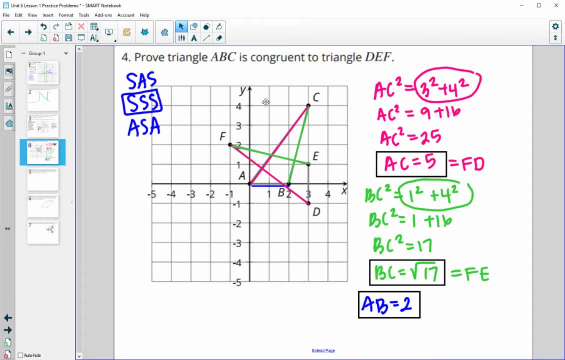 And then when we look at the final side, The final side is vertical, so we can just count it- and has a length of two. So ED has a length of two. So then we've shown that all three sets of sides are congruent. 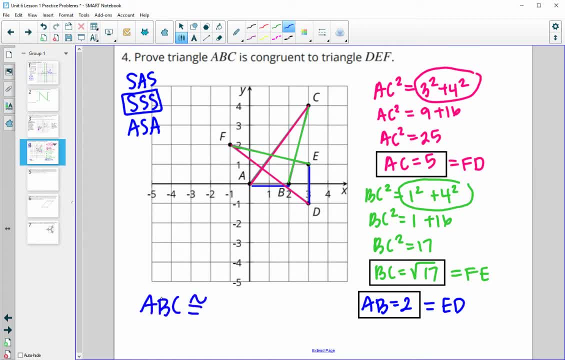 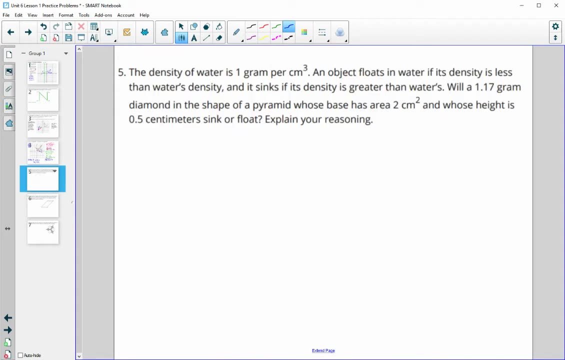 So triangle ABC Is congruent To triangle DEF, By side side side. All right, then density. So for density we do mass divided by volume, So the weight or the mass divided by the volume, And for water, the density. 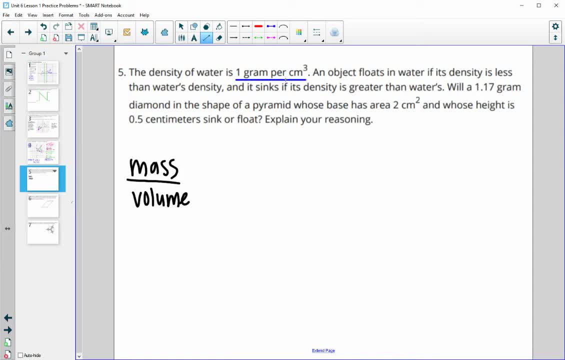 Is water: One gram per cubic centimeters. So if an object has a density less than one, it's going to float, And if it has a density higher than one, it's going to sink. So we want to take a look at this. one point seven, one point one, seven gram diamond in the shape of a pyramid. 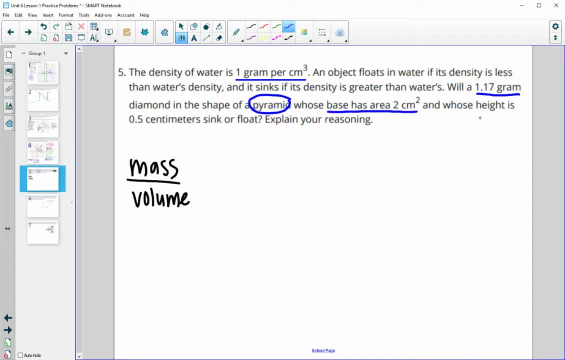 Whose base area is two centimeters squared and whose height is point five centimeters. Will this sink or float? So first of all, we already know the mass. Okay, so we know the mass. here is one point one seven. So that's going to go in for the mass: one point one seven. 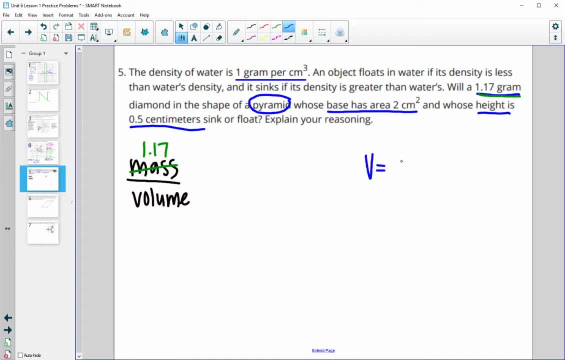 Now we need the volume And we've got a pyramid. So we want to do area of the base times the height, divided by three. So the area of this base, they told us, was two, They told us the height was point five, And then we would divide by three. 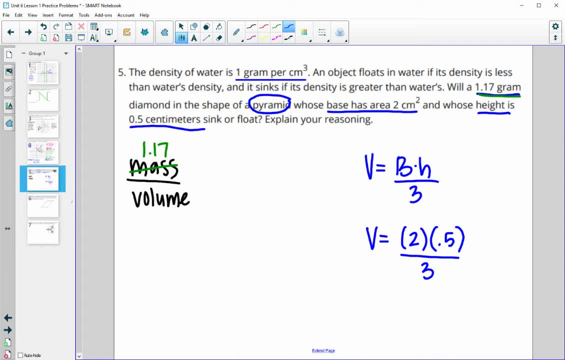 And then we would divide by three, And then we would divide by three, And so when we do that, we end up with: the volume of this pyramid is point three, three, three, repeating, And so that's going to go in for the volume. 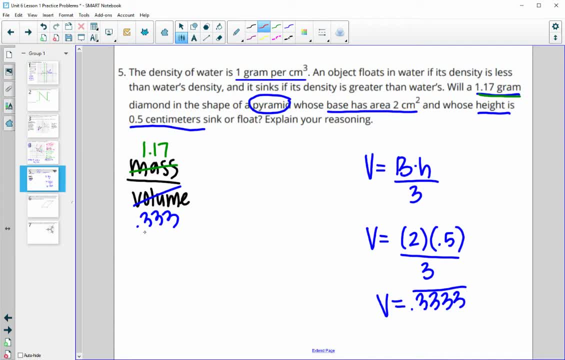 So now you probably know point one divided by point three is going to be bigger than one, because point three is going to go into one more than one time, So this is going to sink. You can also actually calculate it out. So one point one, seven divided by point three. 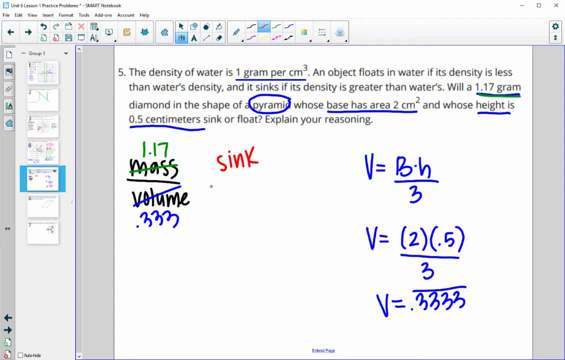 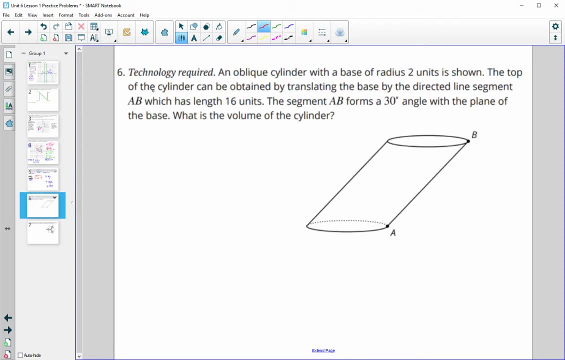 Three, three, three, three gives us a density equal to three point five, one. Okay, Again, that's greater than one. So this diamond is going to sink in the water, All right. Number six says an oblique cylinder with a base radius of two is shown. 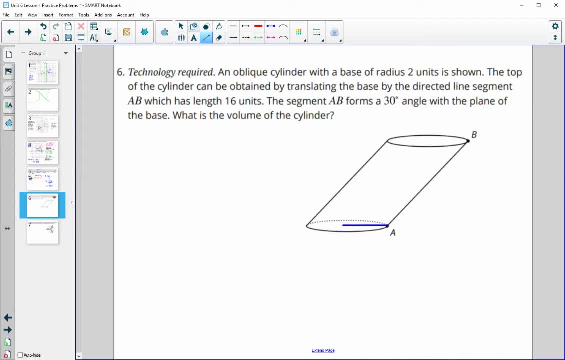 So we know that the radius here of this circle is two units, Or two, Yeah, two units At the top of the top of the cylinder can be obtained by translating the base by a directed line, segment AB, whose length is 16.. So this AB's length is 16.. 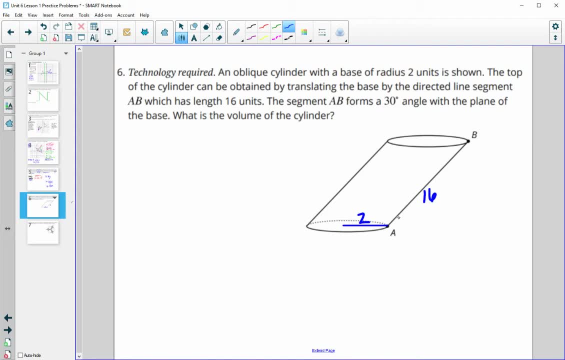 The segment AB forms a 30 degree angle with the ground. So let me get a dotted line here. So this angle formed here is 30 degrees. Find the volume of the cylinder. So we'll need the height of this cylinder, Which it's oblique. 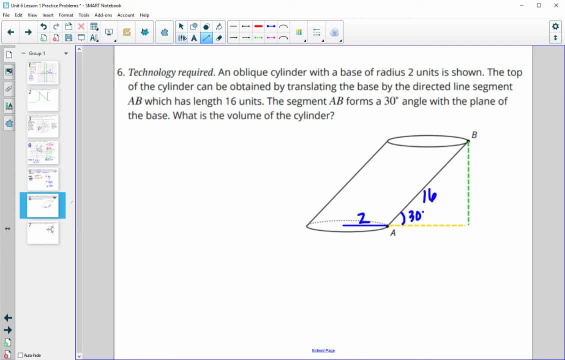 So it's going to be on the outside here, So we'll need to find this height, And there's going to be a couple different ways that we can do this. So first of all, hold on. Let's put in the volume formula for. 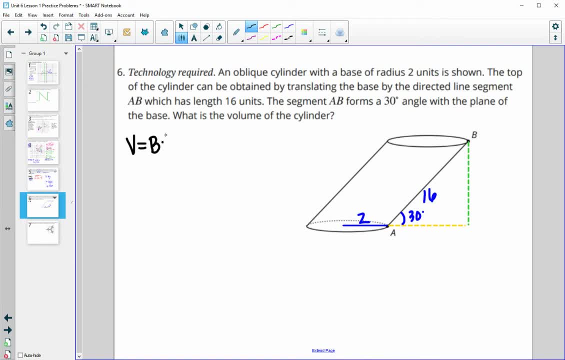 Cylinder is just area of the base, times the height. So for the area of the base we can already find that The base is a circle. So we will just do pi times the radius, In this case two squared. So the base area is four pi. 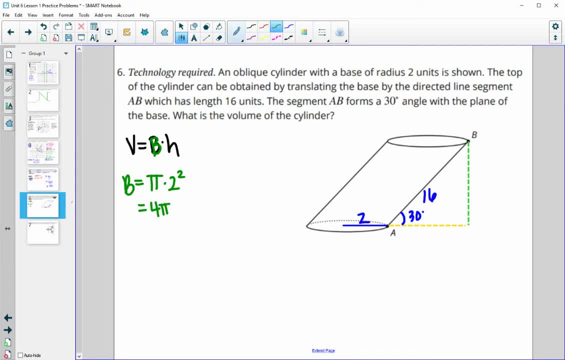 And then we need to find This height here, And so there's going to be a couple of different ways that you can do that. We've got this 30 degree angle. So if you remember your special right triangle formulas, the short leg- 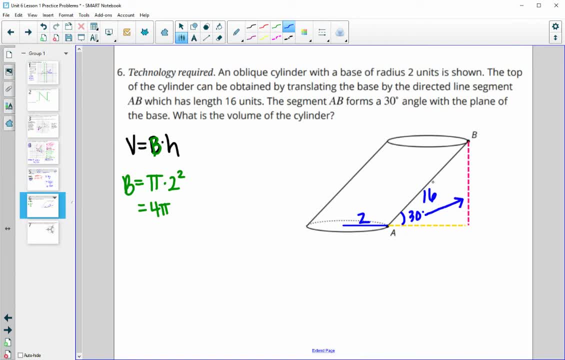 So the leg across from the 30 degree angle is half of the hypotenuse, So this is going to be eight, Since this hypotenuse is 16.. So if you remember that formula, you can certainly use it. You can also set up trig functions. 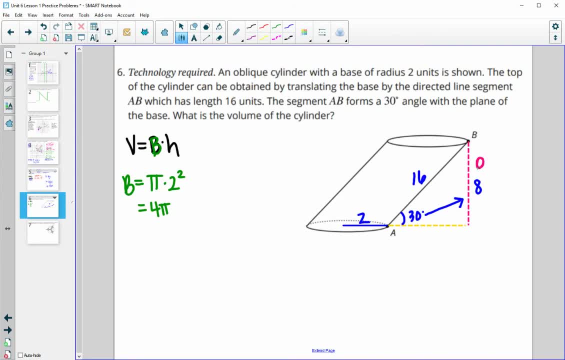 So, across from the angle, which is what we're looking for, is the opposite side, And then we're also given the hypotenuse. So this is a sine function. So we would do sine of 30. Equals the opposite side, Which I'll just call X, over the hypotenuse 16.. 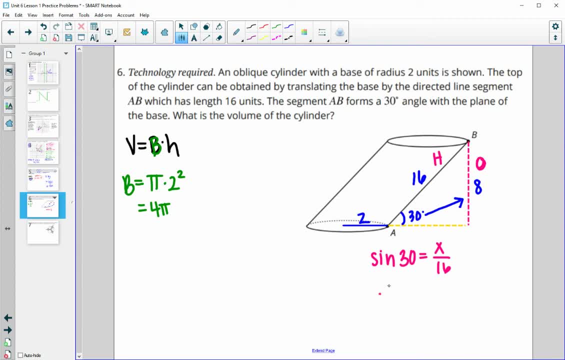 And then you would just use your calculator to do sine of 30. Which you get 0.5. And then we can make this into a proportion And we can cross multiply. So 16 times 0.5 gives you 8.. 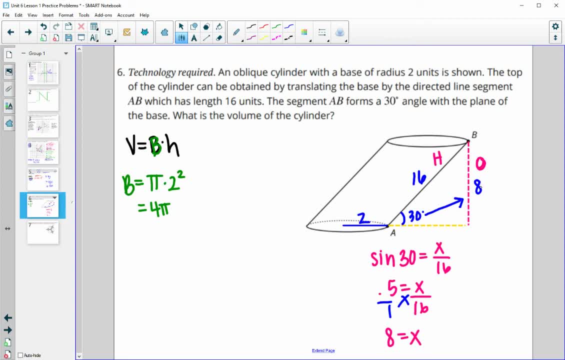 So 30,, 60,, 90 formulas gave us 8.. Also trig gave us 8. So we get a height here of 8. So in this volume formula we will do area of the base times. the height Area of the base again was 4 pi. 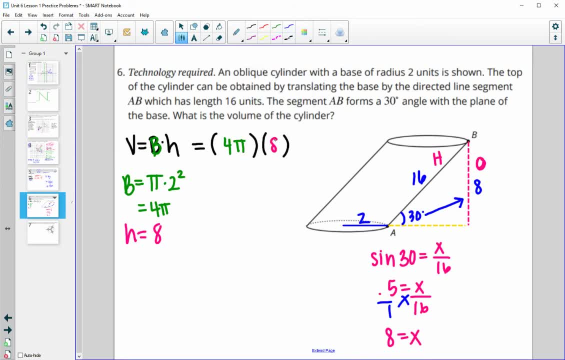 The height is 8.. Multiply those together And we get 32 pi units cubed for volume. And if you actually want to get the decimal version of this, You can multiply 32 times pi And we would get about 100.5 units cubed. 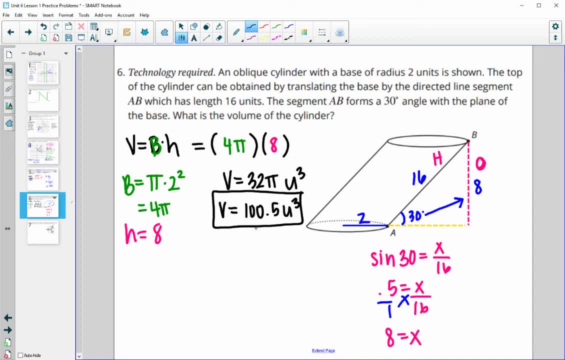 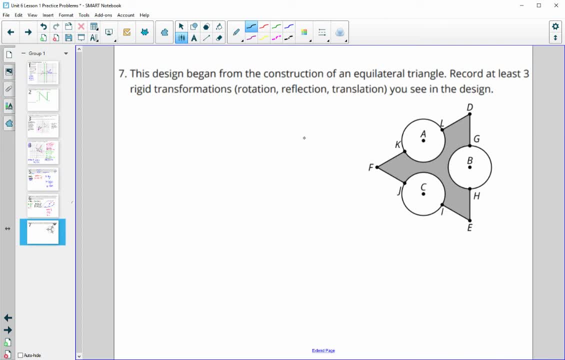 So if you wanted an exact form, 32 pi, If you want decimal, 100.5.. All right, Then this one says: the design began from the construction of an equilateral triangle. Record at least three rigid transformations that you see in the design. 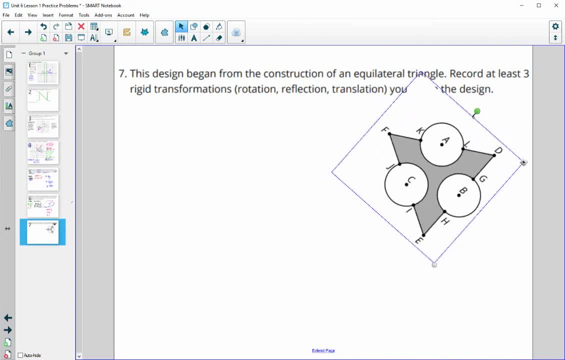 So this has rotational symmetry, So we could rotate this on itself. So let me do this and show you what this looks like. So if you rotate it around the center, This can just rotate back on itself. If we can get it to go exactly around the center, 120 degrees, it would just rotate right back on itself. 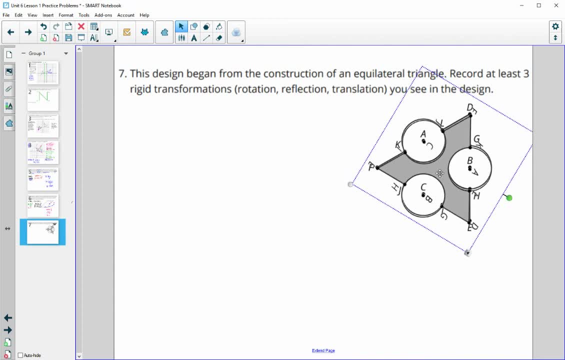 So rotation around the center of the triangle 120 degrees or 240 degrees would work. You can also see that these circles could translate to each other. So if we just look at the circles and not the whole picture, You could translate circle A by directed segment AB. 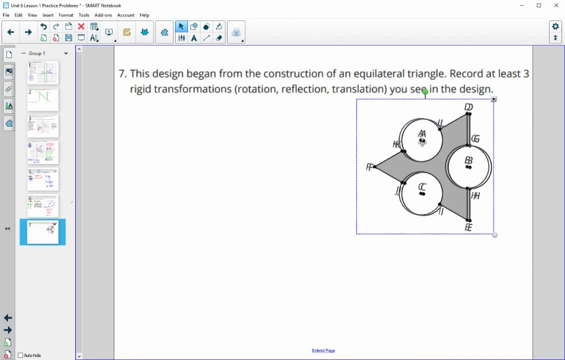 And it would land on that next one. So that would be a type of transformation we see happening in there. So you could take- Let me get rid of the rest of that- You could take this circle And translate it from A to B and it would land there. 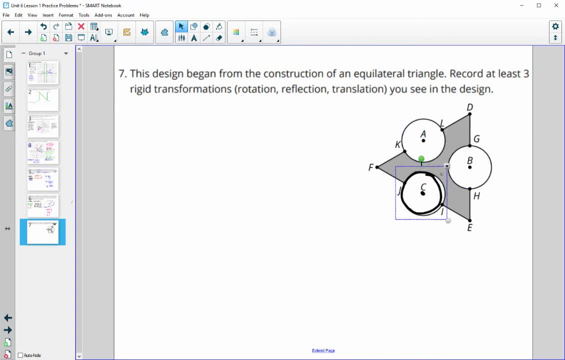 Or you could do it from A to C or C to B. Hey, those would be translations. You could do a reflection over a perpendicular bisector. So if we did like, if we connected these, We could reflect this over the perpendicular bisector. 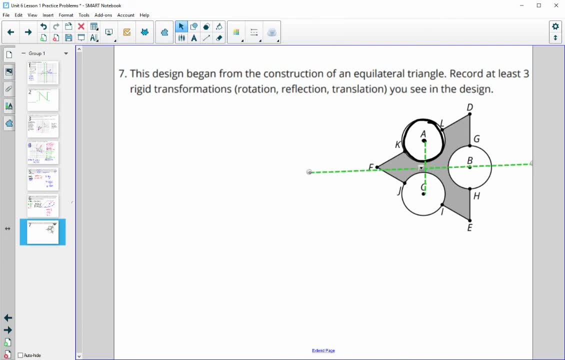 Of that segment, And then it would just fold, fold over itself. So then this top half would fold over onto the bottom half. Could also, could also. maybe I'll use a different color than this Green, maybe something else will show up better. 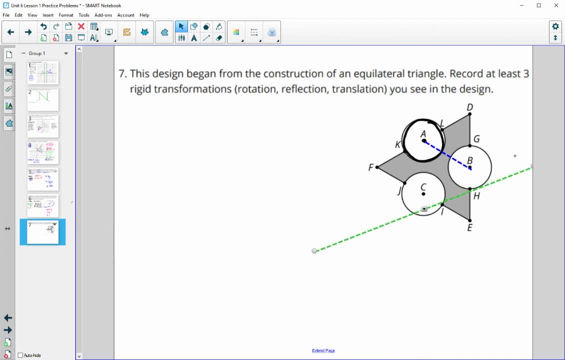 So I could do it over this perpendicular bisector as well, So the one of AB, And then that shape would fold over Again. So reflection over the perpendicular bisector of AB or AC or BC, Rotational symmetry Translations of those circles are just a few that you might have seen. 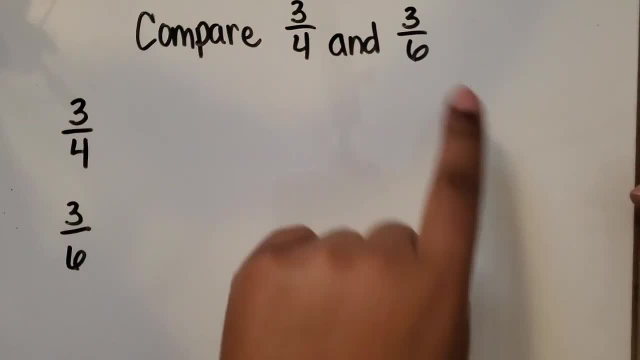 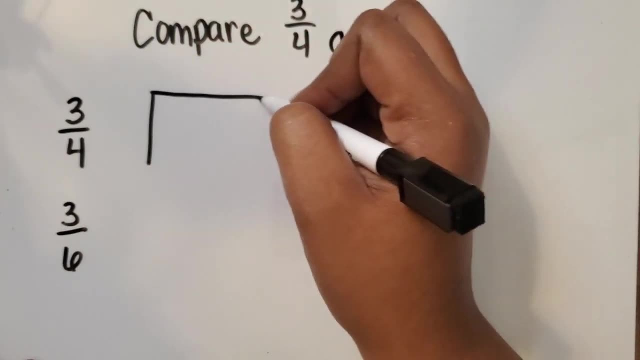 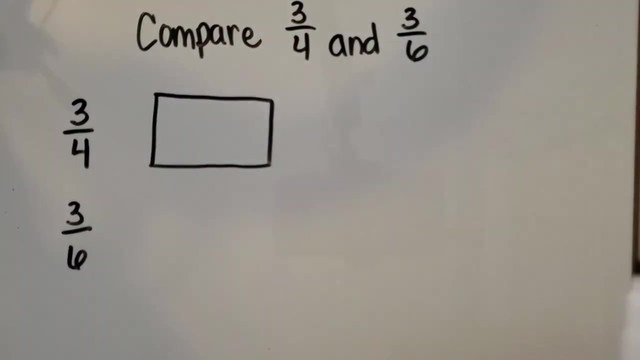 We are going to compare the fractions 3- fourths and 3- sixths using rectangular area models. So first we're going to draw 3- fourths, I'm going to draw the rectangle as a whole, And here we can see our two fractions have the same numerator but different denominators. 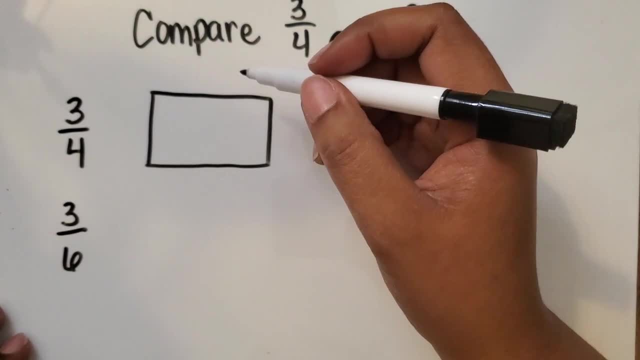 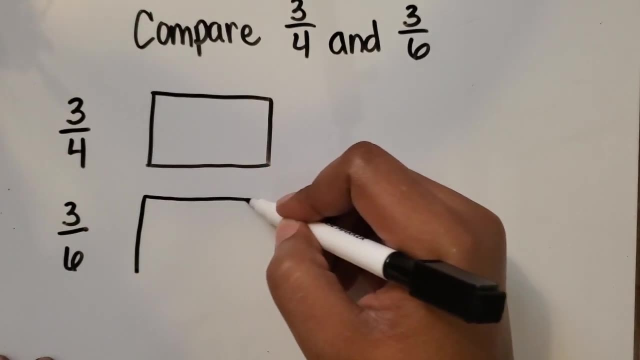 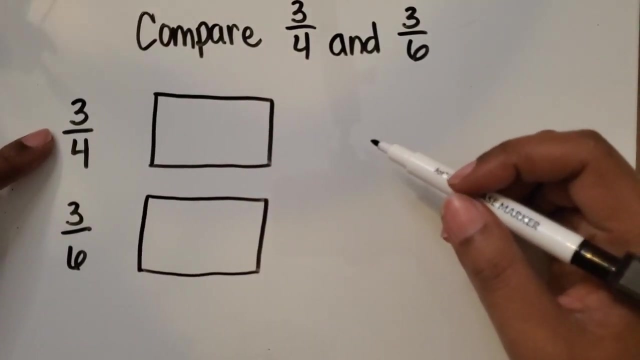 So how we partition or split up the whole is going to look different. So we have one whole and I'm actually going to draw my second whole to make sure I have the same size whole. Okay, so the first fraction is 3 fourths. so I'm going to partition the whole into 4 equal parts.